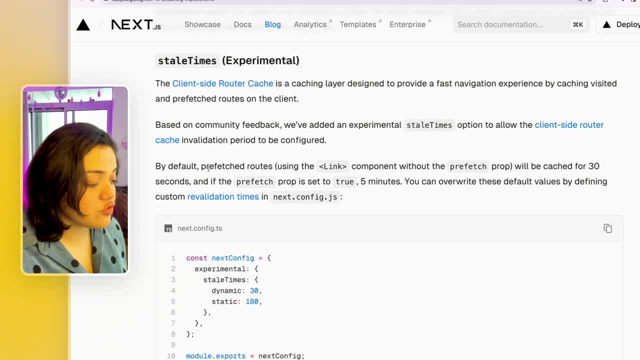 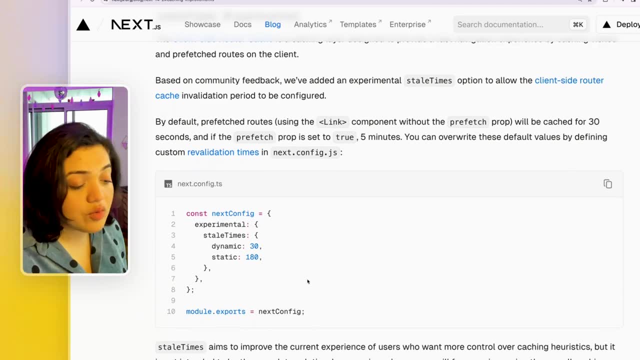 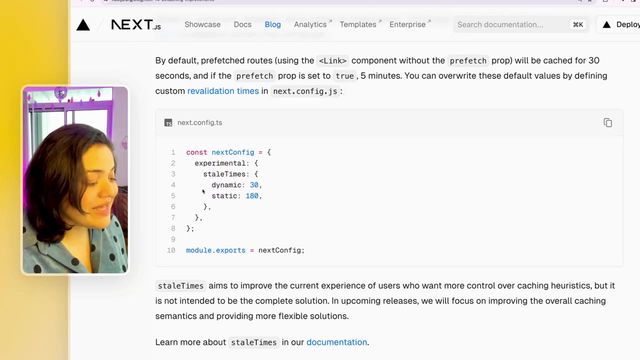 prefetched prop, which is which will be cached for 30 seconds, And if the prefetched prop is set to true, then it will basically be five minutes. And we can completely override these default values by passing in the experimental object inside of the next config file and then adding stair times. 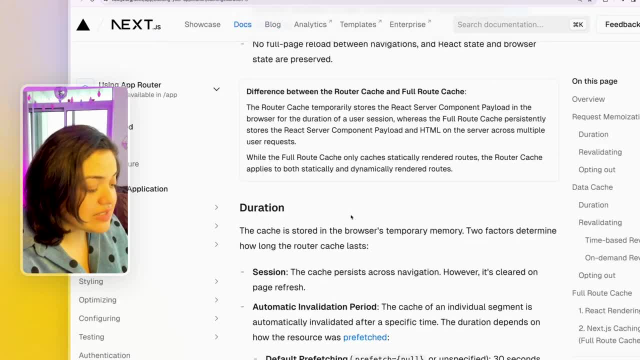 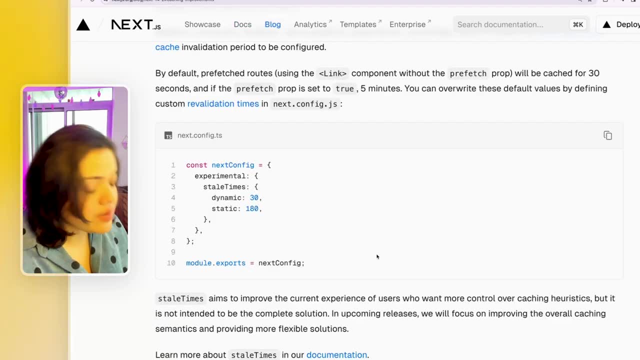 and adding dynamic and static. Now we can easily do that, as they showed us, and the revalidation time and the documentation has also been updated for that. But keep this in mind: that it's completely experimental, So you can definitely try it out, but it's still experimental, So things might. 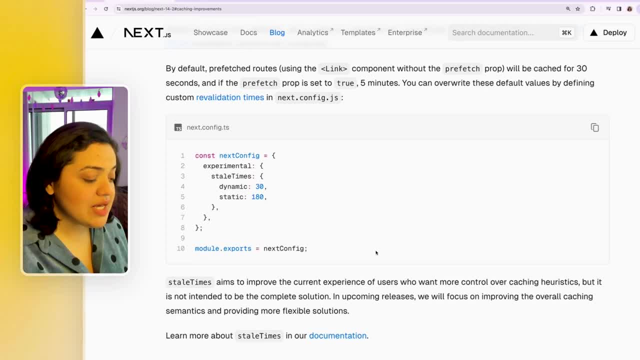 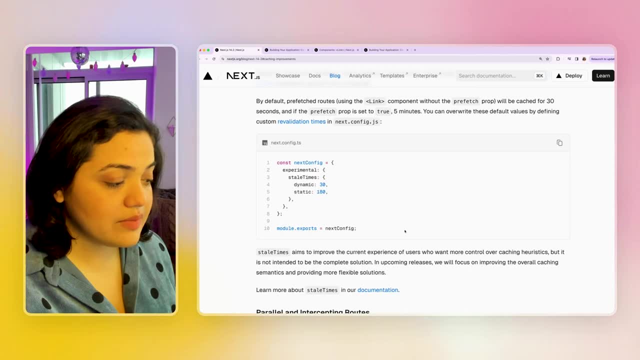 change in the future, But I'm really excited for this specific change as it definitely improves the current experience of the users and we get more control over the caching heuristics. Now, definitely, we are heading in the right direction, as the community has been really. 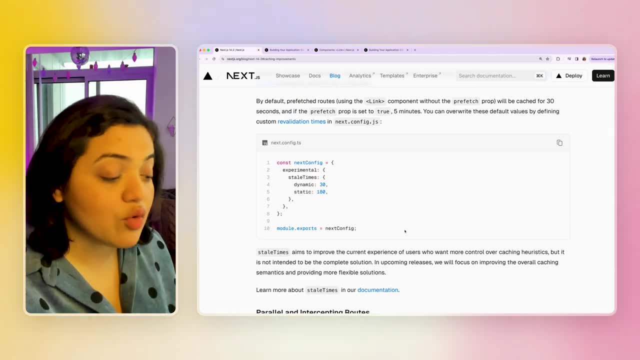 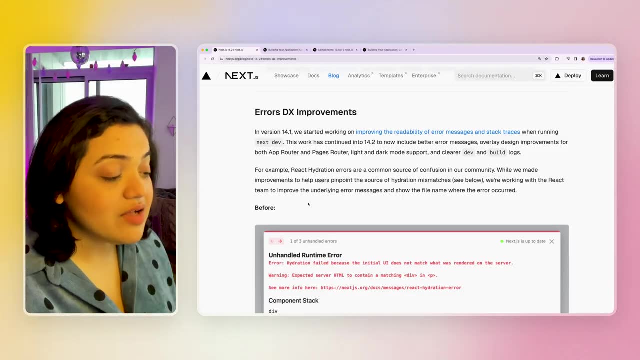 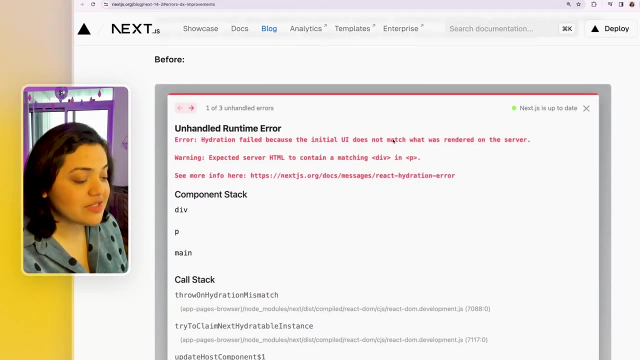 requesting to have more control over caching and more configuration capabilities over caching. So this is pretty awesome. And the next thing that I'm really excited about is the error experience improvement. If you remember, whenever we got this specific message: hydration fail because the initial UI does not match what was rendered on the server. 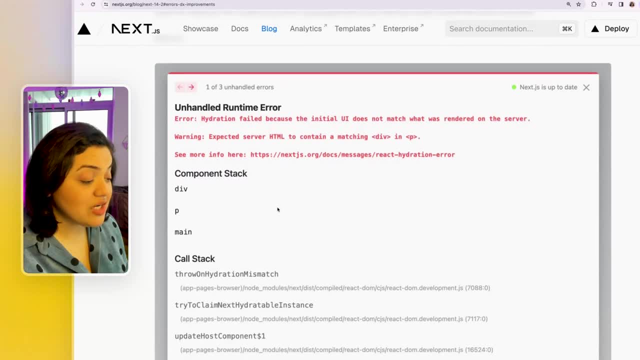 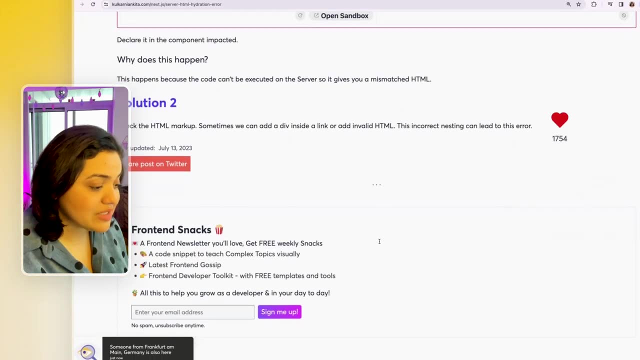 then we would get this specific warning And that's pretty much it. This is the component stack. It would be really hard to figure out why it failed. I do have a blog post on this specific topic as well, where I essentially talk about how you can solve the hydration errors too. 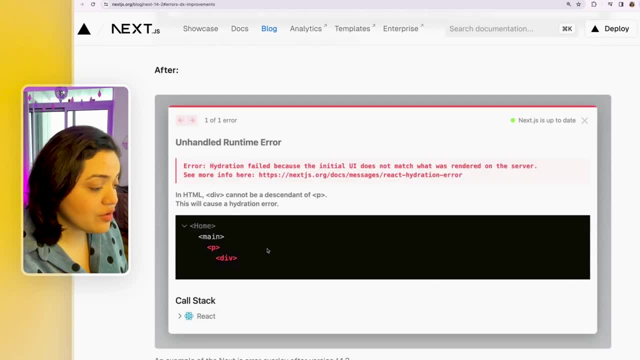 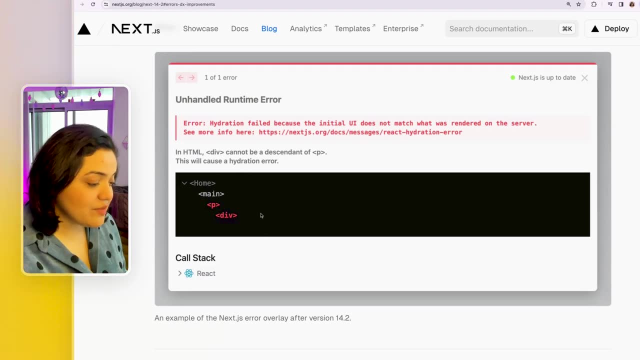 If this is a before photo, this is going to be the after photo, where we would be exactly the call stack And you will know why the hydration error occurred. So, for example, in this case the div cannot be a descendant of p, because sometimes we don't use proper semantics. 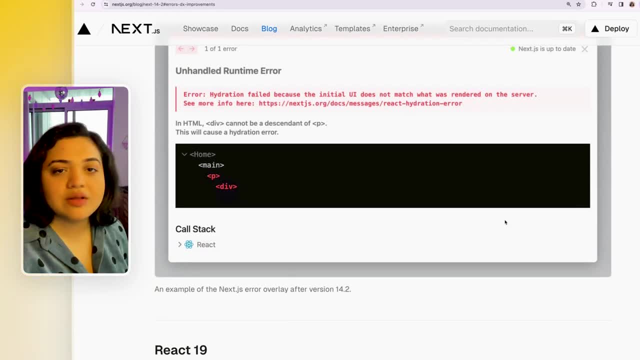 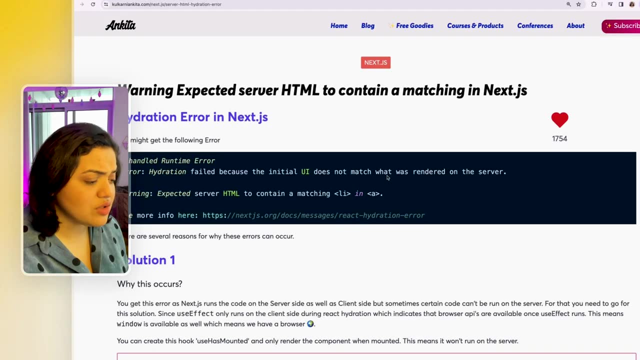 and this can be as a result of that. Earlier, we had to go in the browser console to take a look at why that error occurred or even add additional capabilities, like I've shown in the specific blog post, to add a specific hook, to check if the component has been mounted, and whatnot. But we don't necessarily need to do that anymore. We might in some cases, but I don't know. So we're going to get into that pretty soon, But we don't necessarily need to do that anymore. but we are going to get into that pretty soon, But we don't necessarily need to do that anymore. We might in some. 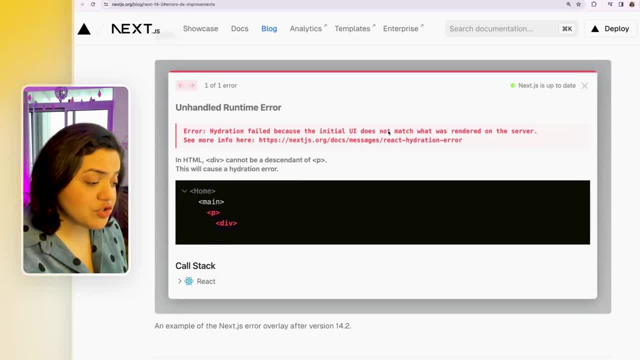 cases, but we're not sure that we're going to get into that. But we faced also the problem. need to do that anymore might in some cases, but but the majority of the cases. if you see the specific error, we know exactly how to fix it and what went wrong, which is pretty awesome, and i'm 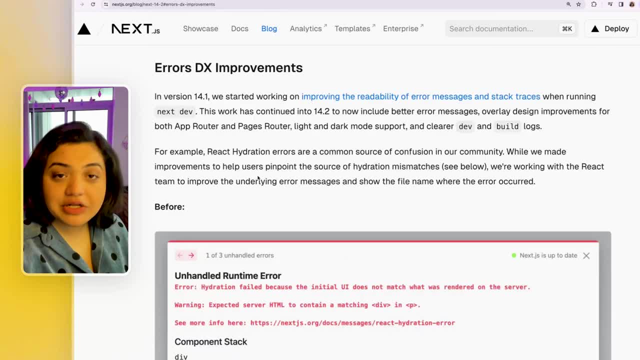 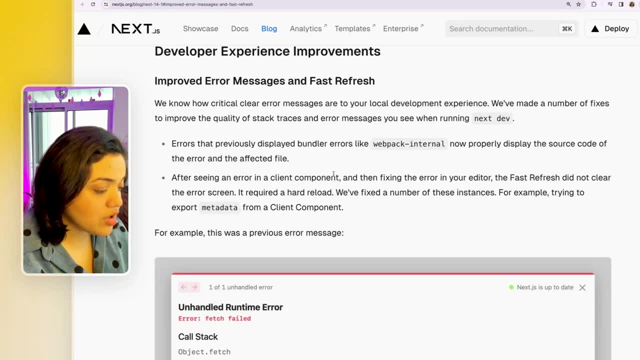 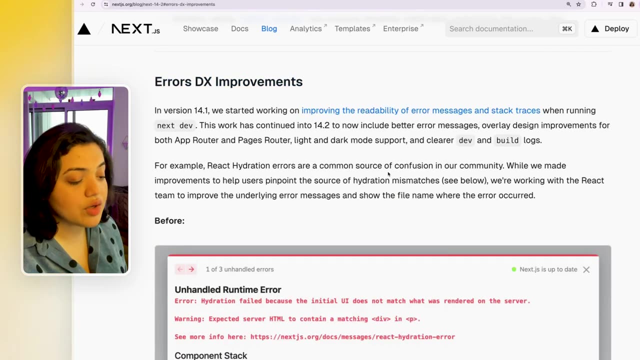 really excited for this, because this is huge. now they are continuously working on updating these error messages as well, so it's really good for us and the previous version. we definitely got quite a few different improvements in error messaging, so this is pretty exciting that they're continuing to work on the overall design improvements as well as improvement of different 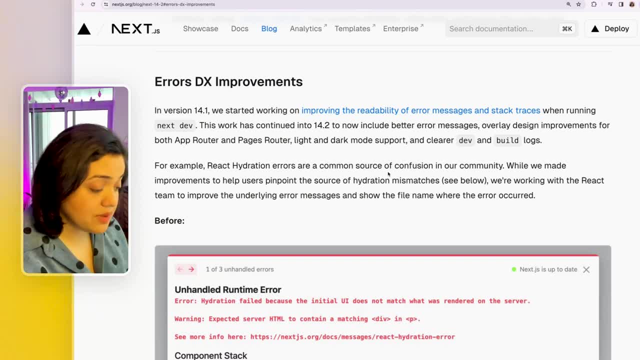 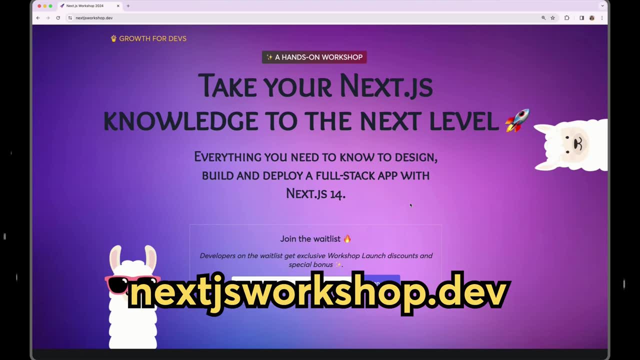 error messages as well, in both the app router as well as the pages router, which is pretty awesome. now, whenever you are ready to level up your next year skills, i have some good news. i'm running a exclusive hands-on workshop for you to take your next year's knowledge to the next level. it will 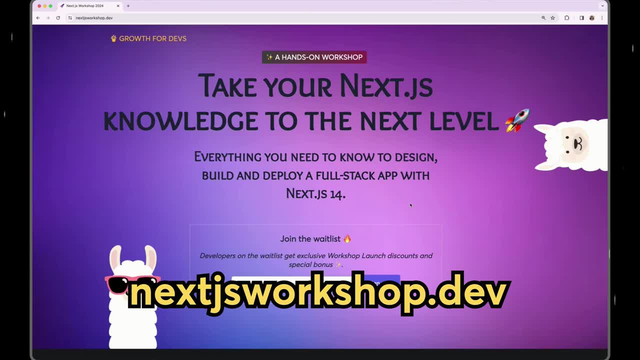 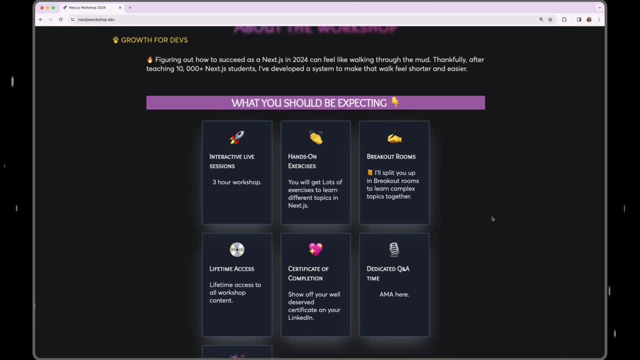 teach you everything that you need to know to design, build and deploy a full stack app with nextjs. it is a live workshop, so you will get direct access to me and i will answer any questions that you may have as well. at the same time, you will get 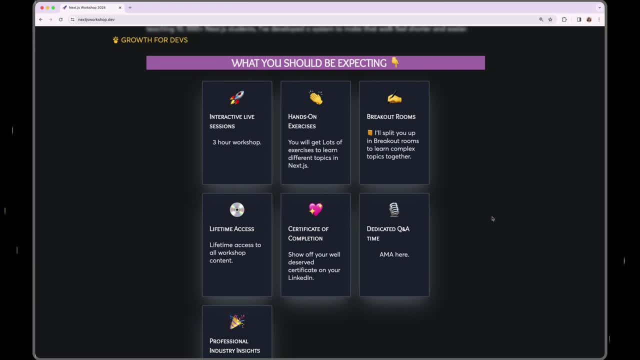 lots of exercises to learn different topics. in nextjs you will be divided into breakout rooms so you can learn from your workshop peers as well and learn complex topics together. and if you get stuck, don't worry, because i'm there to help guide you as well. so if you're interested, please sign. 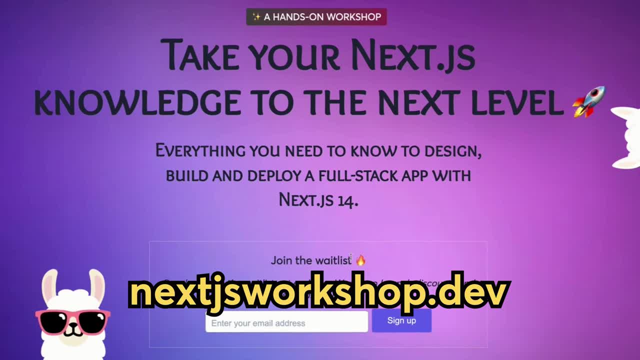 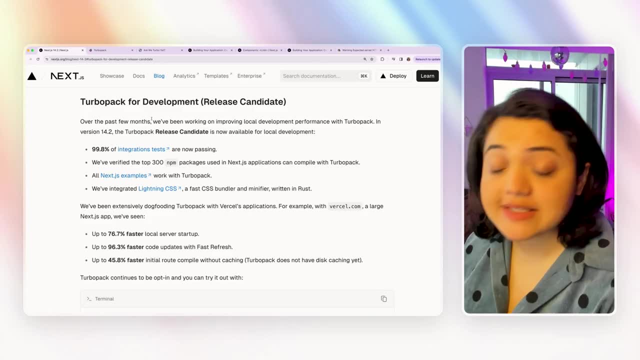 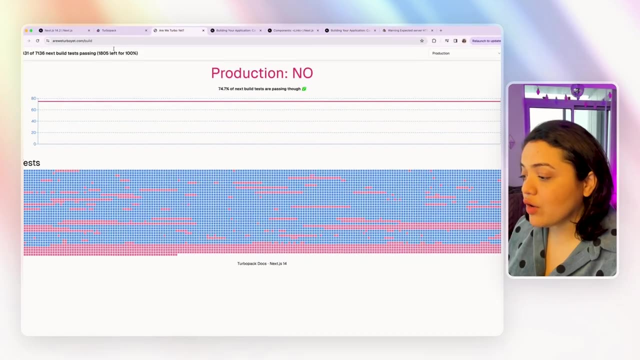 up to the waitlist. as the waitlist folks get exclusive launch discounts and special bonuses as well. the next improvement that's really, really exciting is that turbopack is finally available for development now. keep this in mind: it's not ready for production yet. it is available for development now. if you don't know what turbopack is, turbopack is essentially 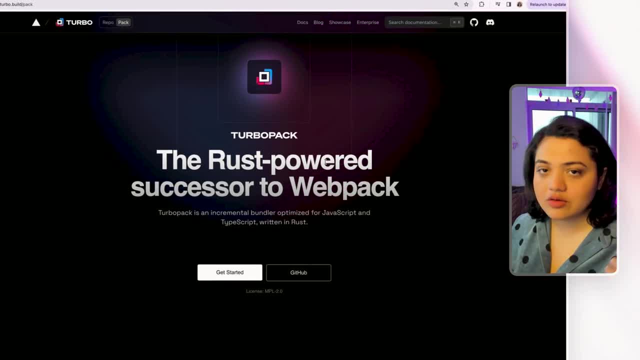 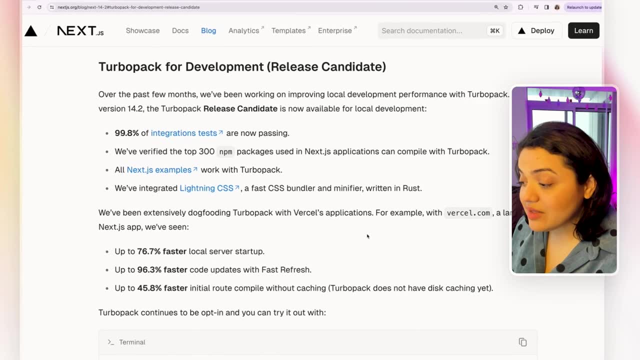 the rust power successor to webpack and it is a really powerful bundler that will bundle all your javascript files and typescript files written in rust. now the fact that they have made turbopack available for development is huge. that means we can start testing it and using it for development. 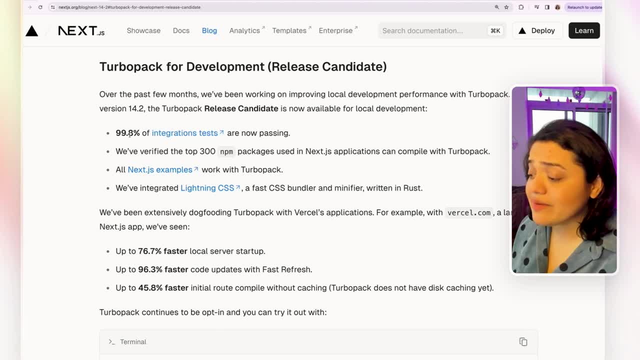 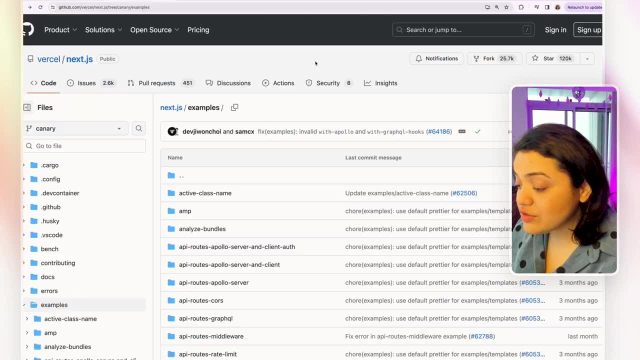 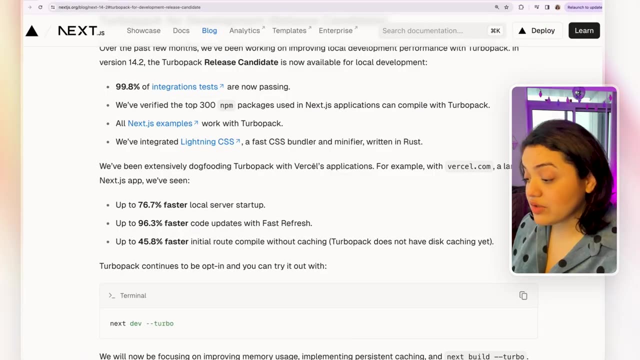 reasons. now the good news is that 99.8 percent of integration tests are now passing. they have verified it with top 300 npm packages. all the next year's examples that they have shown here, they have provided to us, are in fact tested with turbopack. so they work with test turbopack and they have also integrated. 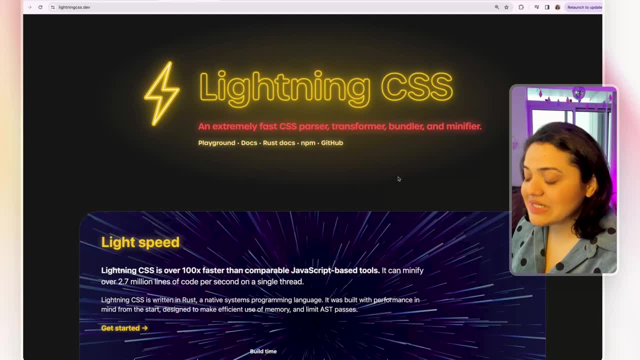 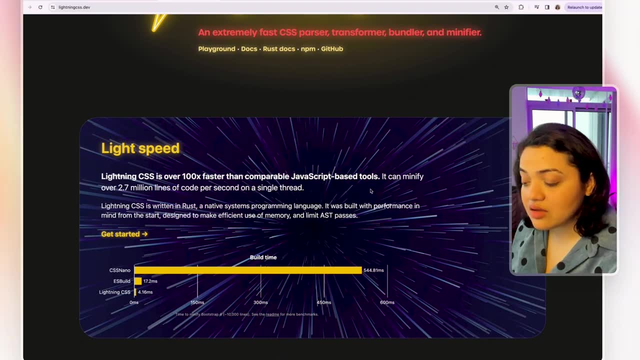 lightning css. now. lightning css is again a really fast css parser, transformer, bundler and minifier. it is 100 times faster than other javascript files and typescript files. and typescript files are now available in the javascript tools. so, for example, if we were to compare lightning css build time, 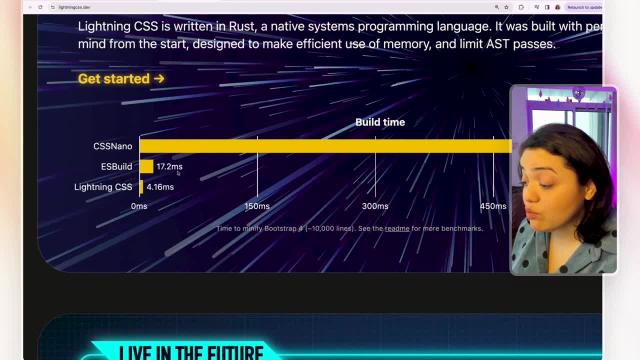 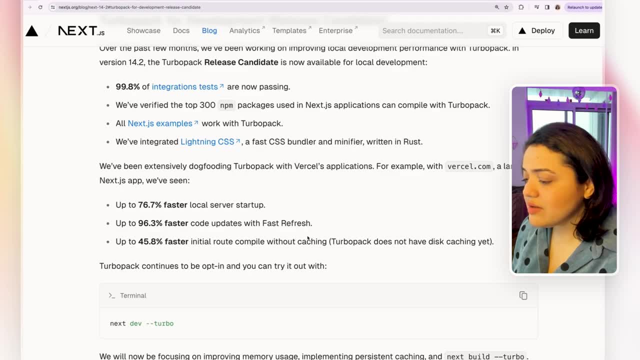 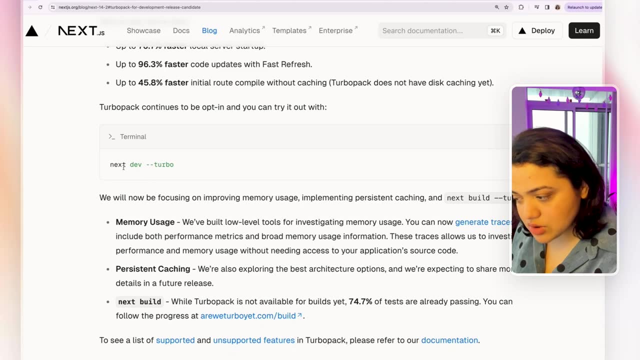 will take 4.16 millisecond. then esbuild is 17.2 millisecond if we were to compare the two, which is really fast. again, it is also written in rust. so the fact that the integrated lightning css with turbopack is definitely the right move because it makes turbopack faster. now we can use turbopack by 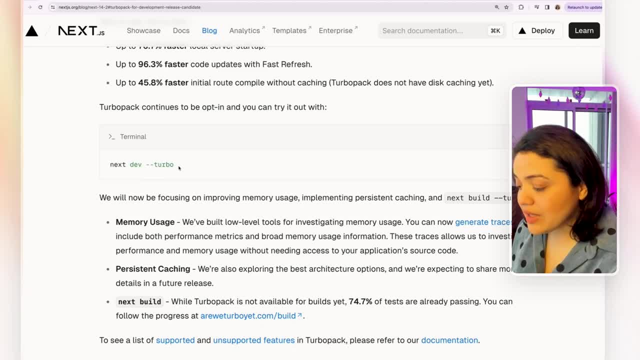 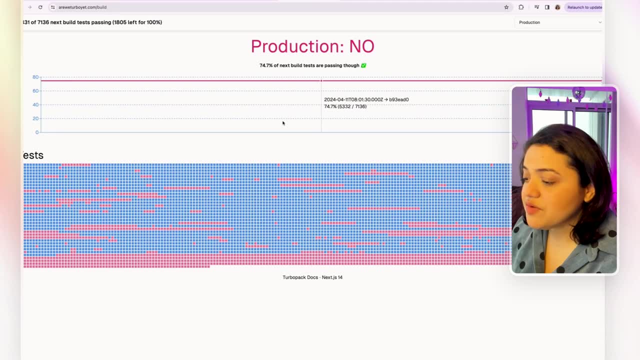 using the option next step, hyphen, hyphen, turbo. and what's really cool is that they have also added a new link for us, which is rb turbo. yet this specific link tells you when it's ready for production. right now. it's a hard now, but they're very close, as 74.7 of the next build tests are. 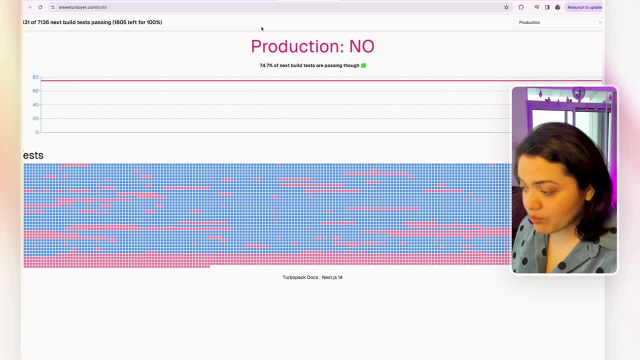 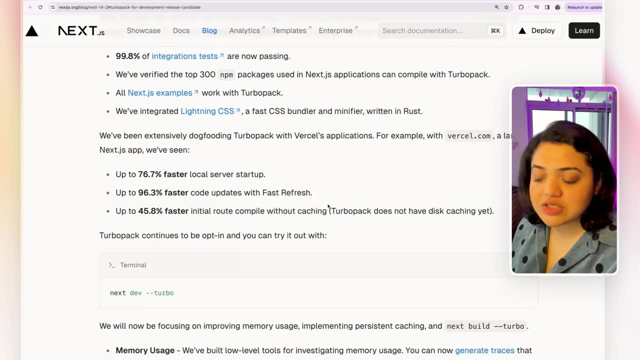 passing through, but again, they still have a bit more work to do, so it's not ready yet. but you can definitely use it for development, which is pretty awesome. so if i were you, i would start testing it out, start playing around with it, but don't use it for production yet. 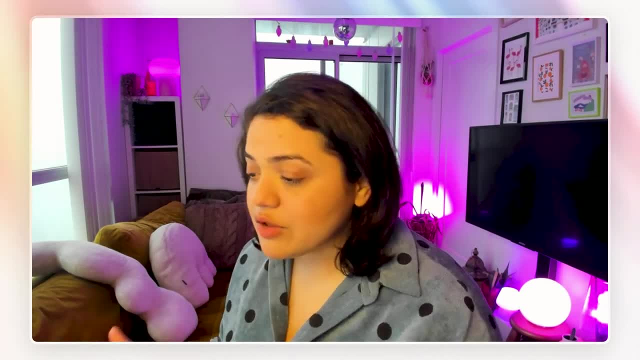 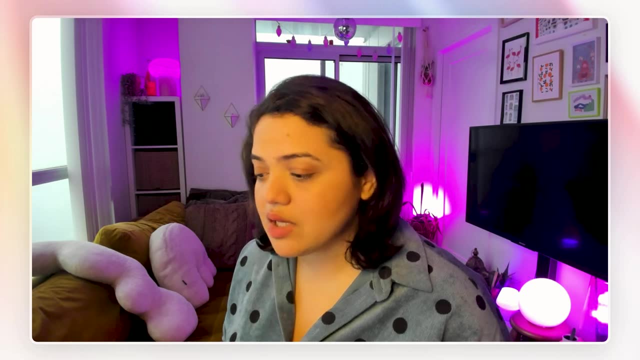 because it may slow down your application or may not. because, again, it is only available for development, not for production yet, and there's a reason for that. but they may discover new bugs or things that may store on your applications. you really don't want to use it for production yet. 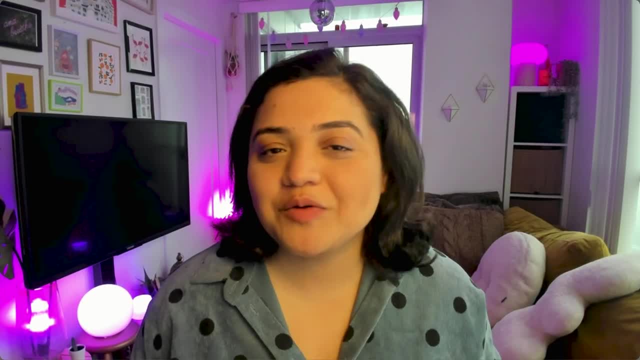 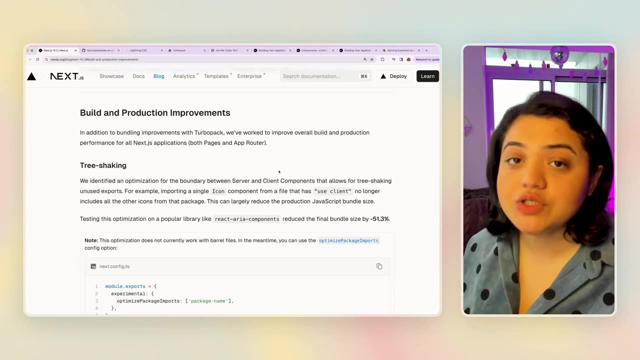 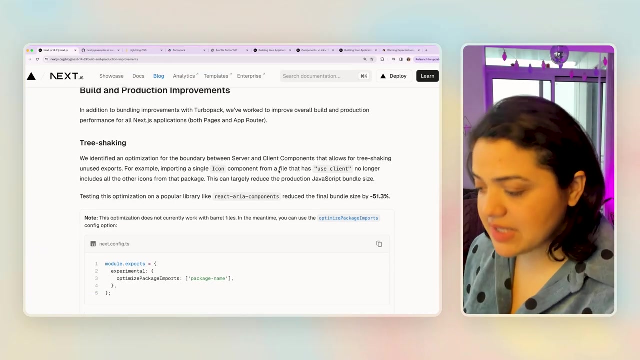 now. if you're enjoying this specific video, now might be a really good time to hit the like button and subscribe to my channel. the other change is the build and production improvements. now, overall, you should see some difference between the previous version and this version, because this is a lot faster now. for example, one of the features is tree shaking. now they have basically 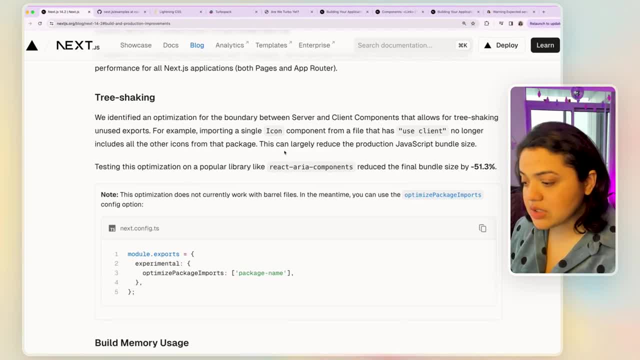 identified the optimization between server and client components. so what used to happen is that, let's say, you were to use a popular library like react aria components, and if you were to import a single icon component from a file that has a loose client, for example, this also would mean that all 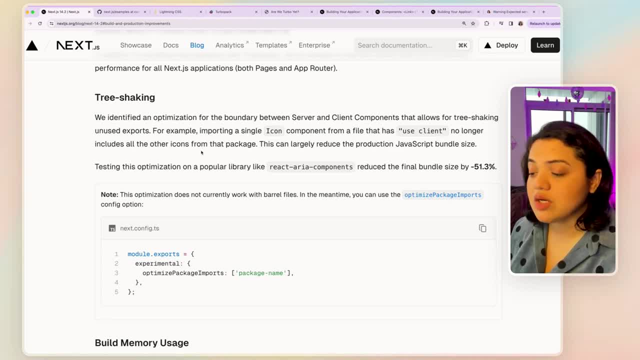 the other icons from that specific package would also get imported from the client, so you would import it in the production bundle, which is not what you want. you only want icon in that specific case and a lot of libraries do offer this specific option, but using the specific use client directive. 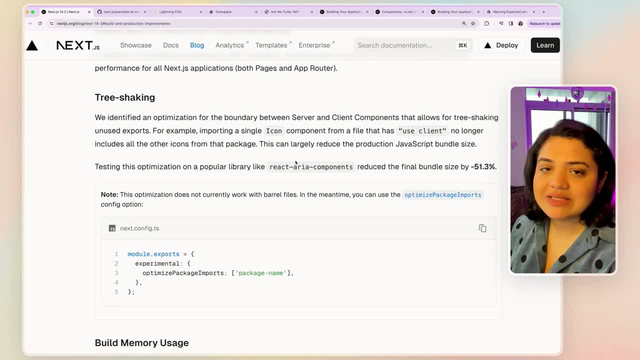 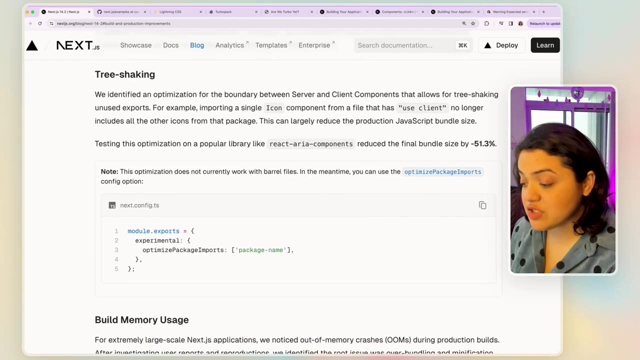 definitely change things at the time, but now they have tested this specific optimization, all the other icons which are unnecessary won't be included in the production javascript bundle, which is pretty awesome, and this means that it reduces the final bundle size by 51.3, which is pretty awesome too. but again, this is also experimental, so you can add the specific flag. 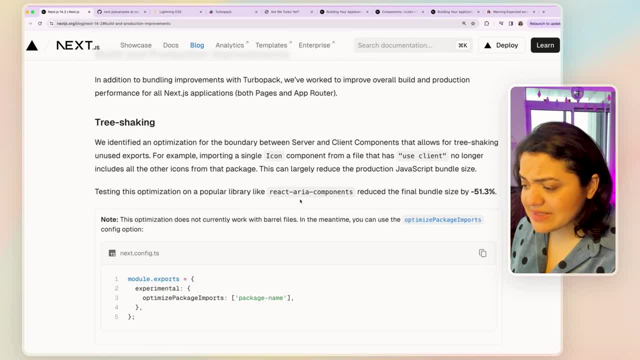 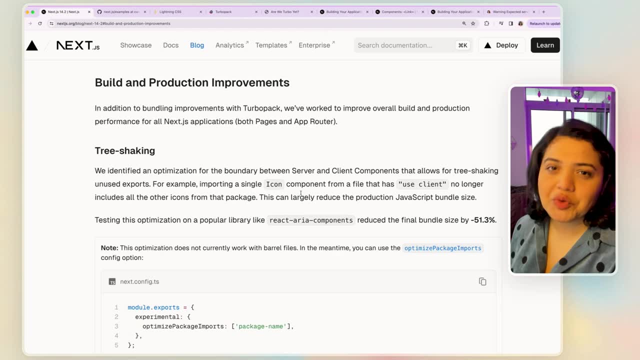 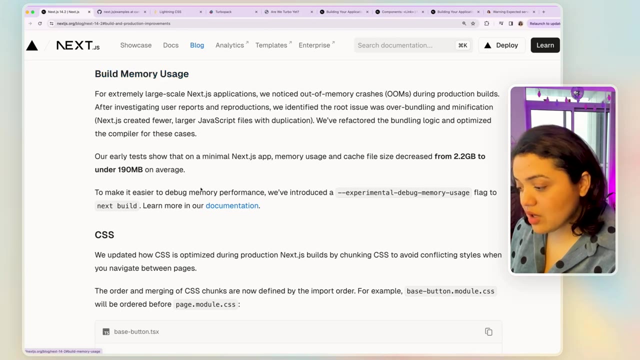 inside of inside of your next config file, to basically test out the specific feature. but this is huge because this leads to improved build time. overall, your production bundle is going to be smaller, which is the goal anyway. then the second one is the build memory usage. what's really? 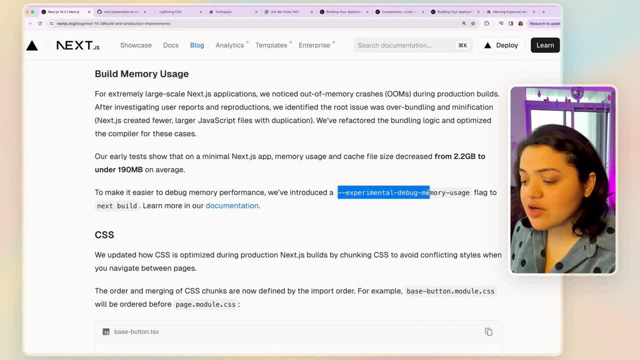 exciting to me is that they have introduced a specific flag called as experimental debug memory, which essentially will make it easier for you to debug memory performance. now, as your application grows so many different files, there might be certain areas where you can optimize your memory and reduce your overall cache file size, and so on. the fact that they have 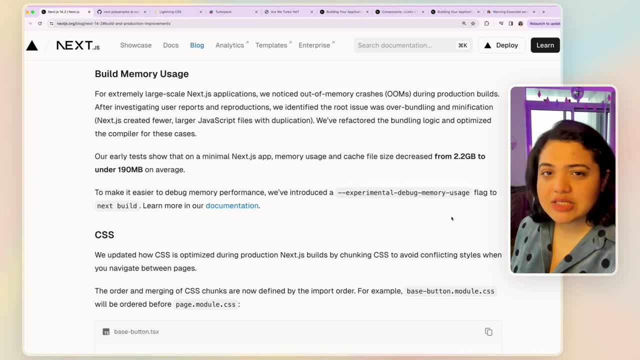 introduced, this specific flag is again paired with caching stale times. i think this is really good because you can now debug out of memory, crashes and so on during production bills. if the experiencing certain errors, then you can basically add this specific flag as well to monitor if it's because of out of memory or just in general overall debug the memory. 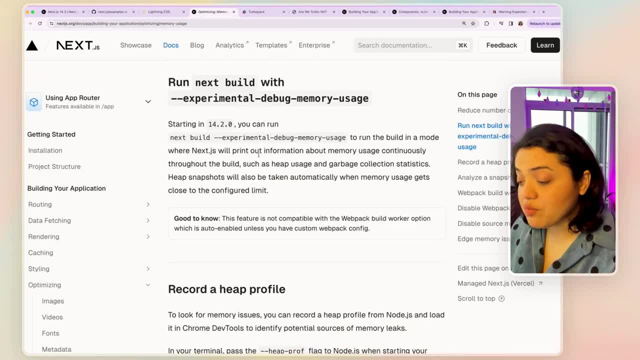 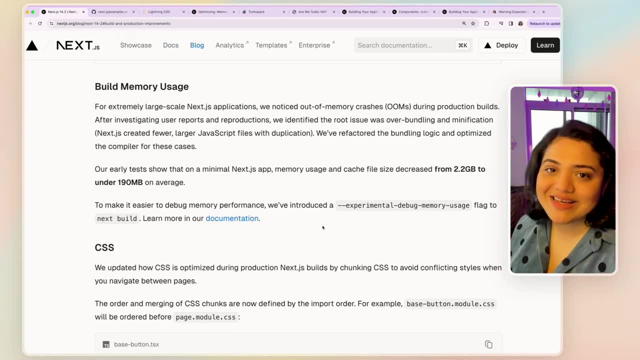 performance as well. so they have provided a lot more information in this specific document that you can take a look at. so this is pretty awesome that we have this specific option. we can debug our next year's memory for our next year's application further. then we also